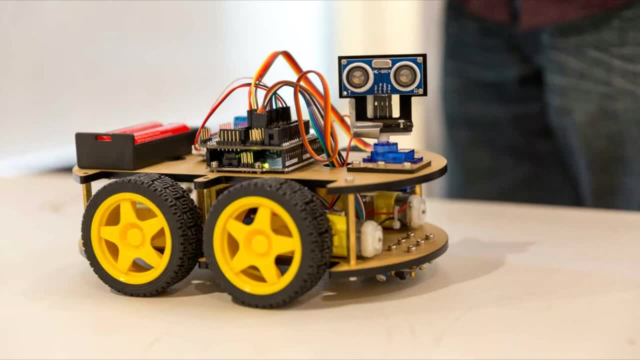 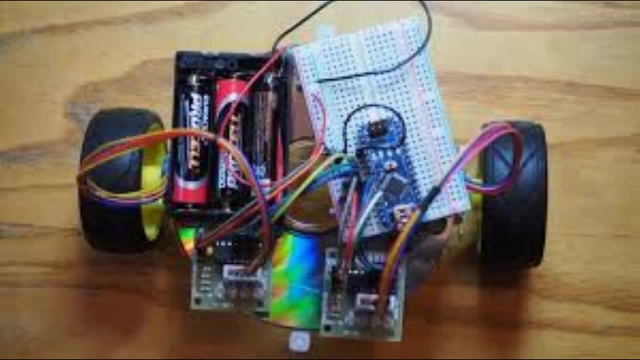 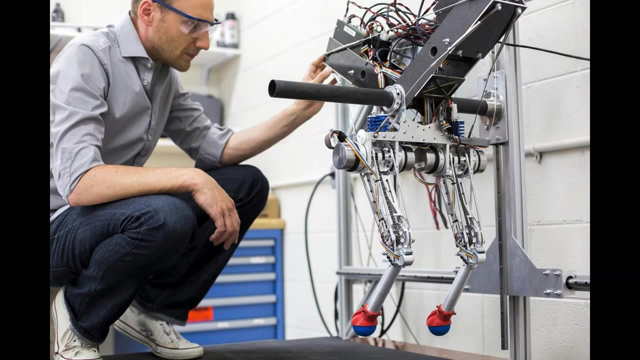 how to use sensors, how to use actuators and how to basically code in microcontrollers, or how to code microcontrollers or how to code controllers, to use sensors and actuators to drive a mechanical mechanism. so that's course number one. it's very critical. you must take that course if 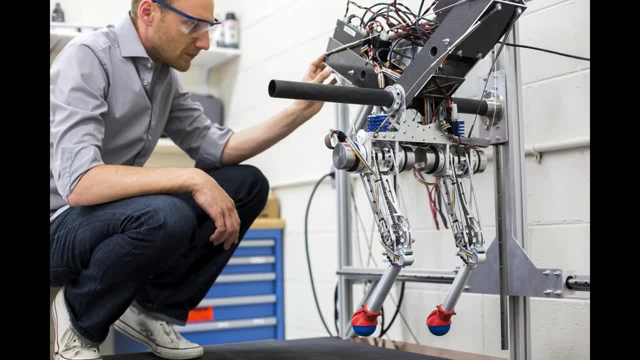 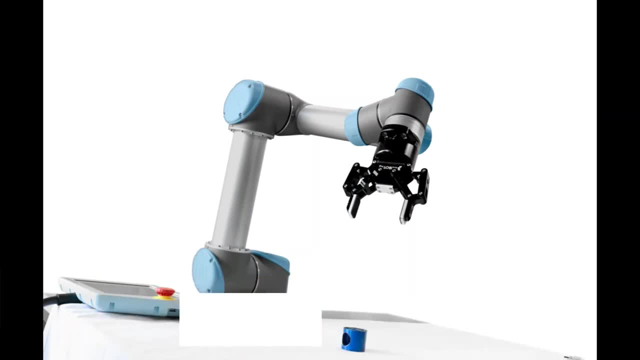 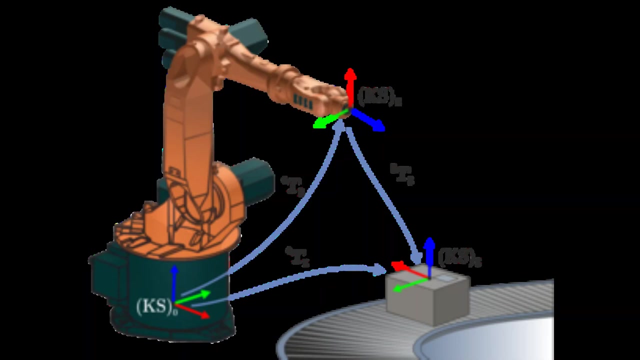 you want to become a robotics engineer. course number two is robotics. so, as the name implies, in robotics you will learn all about forward kinematics, inverse kinematics, how to basically transform between different coordinate systems and, for example, let's say you have a robotics arm and the TCP the tool. or let's to simplify it, let's say like: 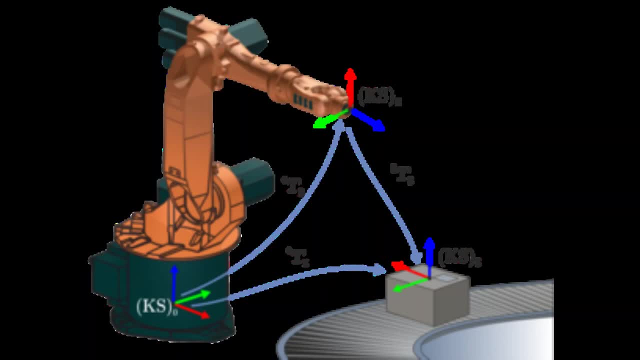 the last joint of the robot. you want to know where the last joint is with respect to the base of the robot, so you need to do a lot of transformation of the robot. you want to know where the last joint is with respect to the base of the robot, so you need to do a lot of transform. 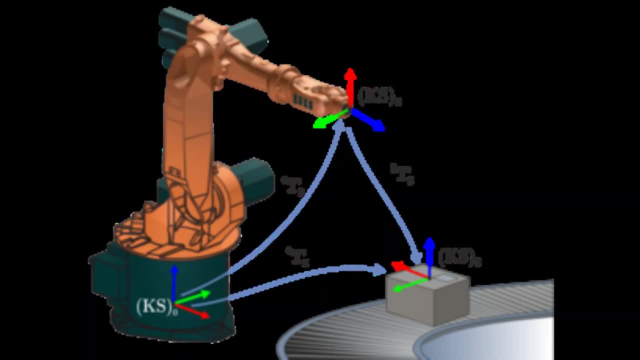 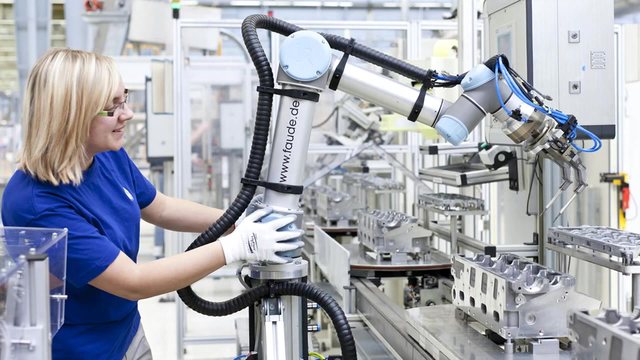 calculation, a lot of different coordinate system transforms. so that course will basically teach you how to basically do all of these transforms and then what forward kinematics mean, what inverse kinematics means what, why you need to learn like kinematics and all about basically robotics. so that would 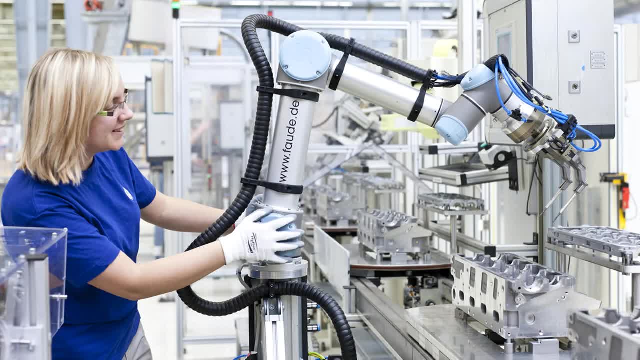 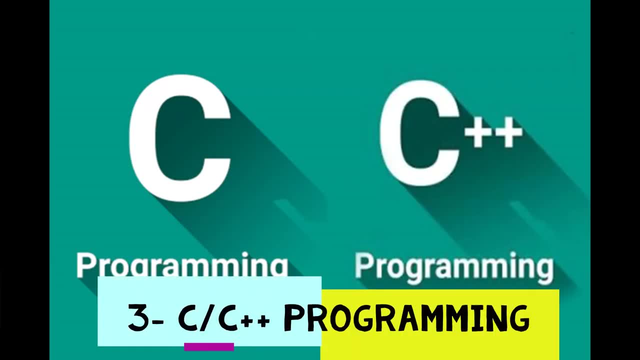 be course number two, that if your college or if your University offers you need to take that course, course number three. course number three is programming in c or c++. as I discussed previously, c and c++ is the best programming language used in robotics, so you must know or you must learn c and c. 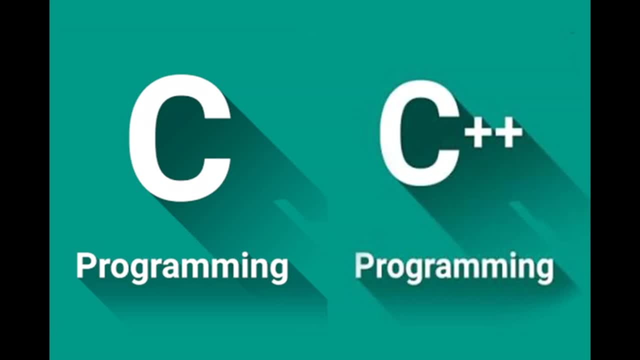 plus plus. you need c and c plus plus, as i mentioned, for mechatronics. you need that to be able to program microcontroller, to be able to program microcontroller to the able to program microcontroller to the program actuators, sensors, and so it's a, it's a must-take course if you want to land a job in. 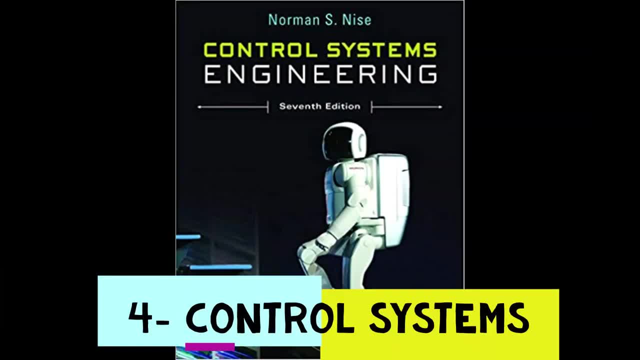 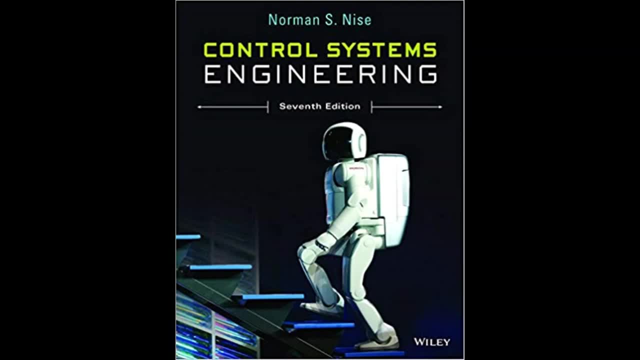 robotics, course number four is control systems. so, uh, you know, in in every robot, every robot, every robot has, uh, some sort of actuators, right, usually it's a, it's a electric motor, uh, and maybe it's a hydraulic pneumatic, but it's usually an electric motor that drives. 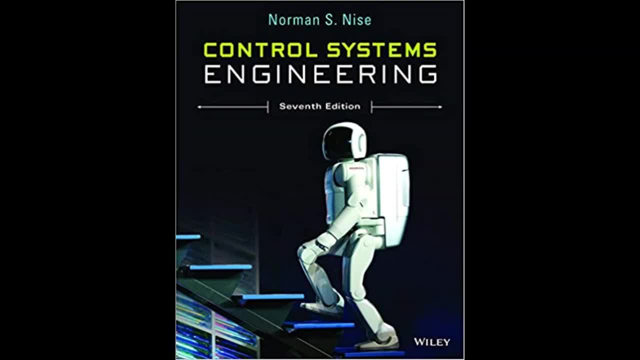 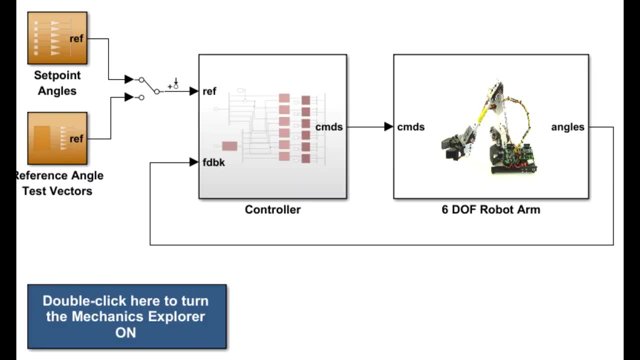 the joint or it drives the mechanism of the robot. so you need to basically able to do position control. you need to be able to do- uh, i don't know- force or torque control or speed control. so if you take control systems then you will learn how to control motors. 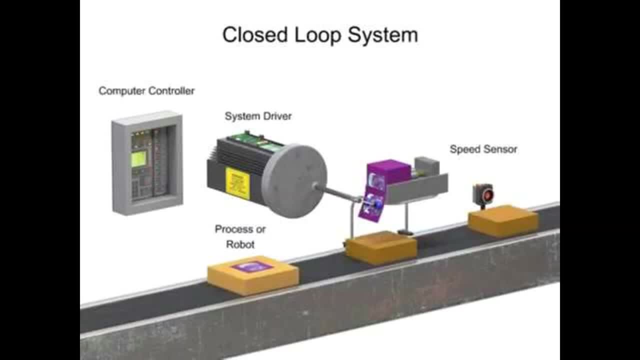 will learn how to implement a pid controller for position control, speed control, force control- so control systems is another must-take course if you want to become a robotics engineer or if you want to land a job in robotics. course number five: computer vision. it's computer vision. 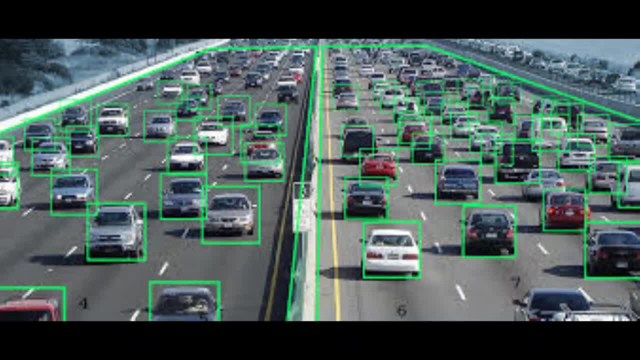 or image processing. that's another course that these days will be very, very helpful, basically doing a robotics project or helping you to land the job in robotics. so almost all the robots have some sort of vision, so it's have some sort of camera or a webcam or something that. 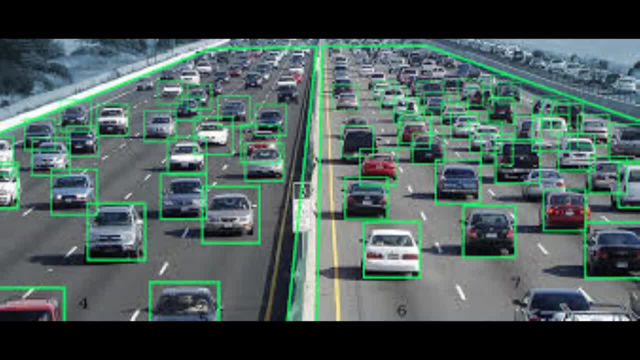 basically, uh, uh, help the robot to to uh, to plan motion or to recognize objects to avoid collision. so, uh, computer vision, it'll teach you all about, uh, images. it'll teach you all about, uh, uh, how to basically segment images, how to recognize objects, uh, and it's a very useful 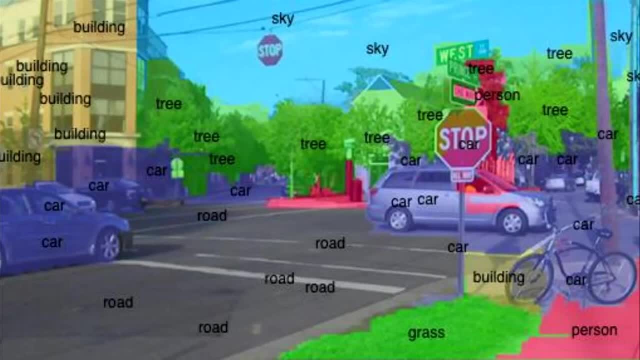 course and uh. usually the computer engineering department or the saw the electrical engineering department. they offer this course and uh. so if they offer to just jump right on it and then take that course, uh, believe me it'll. it'll help you a lot in your future job, or even just.